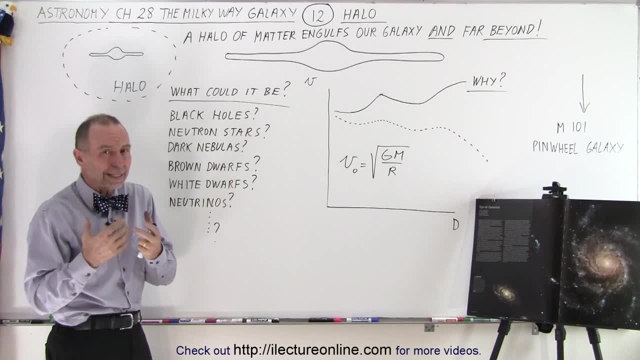 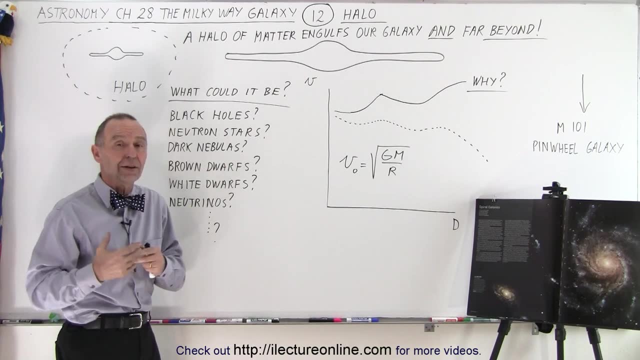 small little ball the size of the Earth, and at great distances they simply cannot be seen because they're not bright enough, they're not big enough. Or maybe there's just massive quantities of neutrinos out there because of their vast quantities. maybe there's much more mass out. 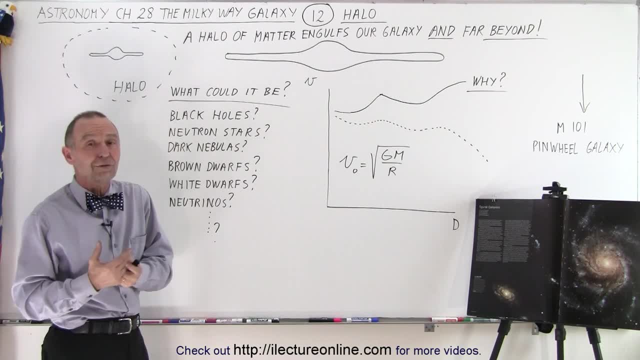 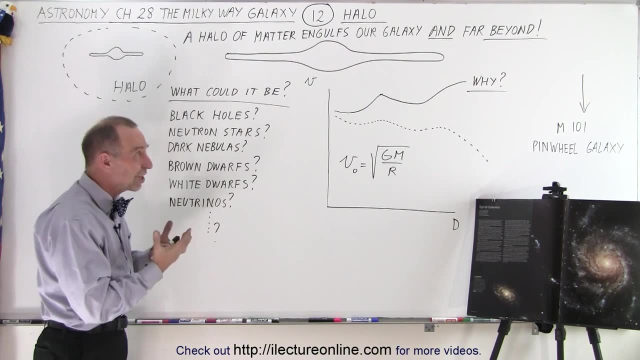 there, at the far reaches of a galaxy that we cannot otherwise account for because it cannot be seen. we cannot detect them. So we've done a lot of studies of all these various possibilities and in each case we've found that there are a lot of stars that are not bright enough, but they're 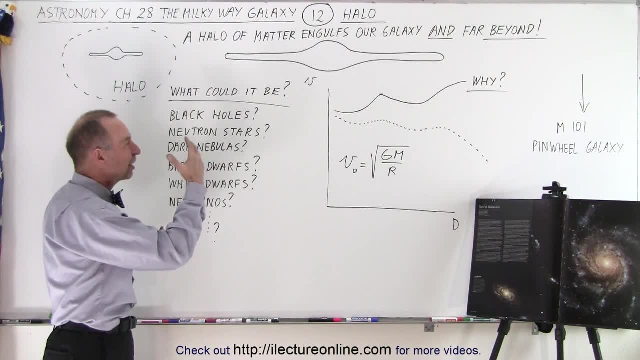 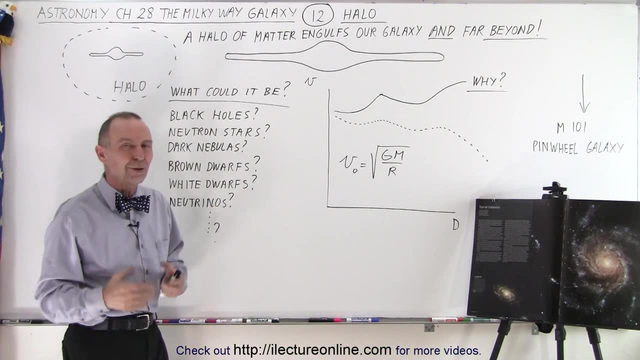 there simply wouldn't be enough of them to account for that additional speed. In other words, there's too much mass here not accounted for. that doesn't fall in any of the categories. There must be something else that's driving the speed of those galaxies because of the additional mass. 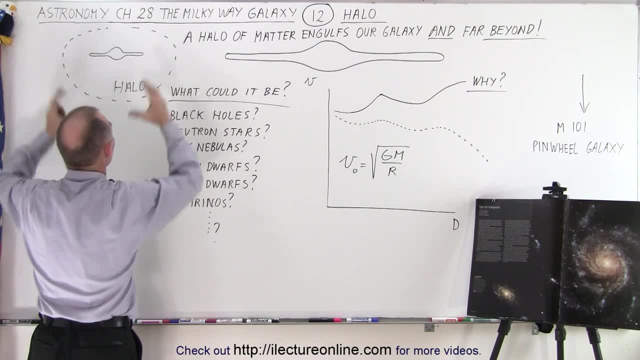 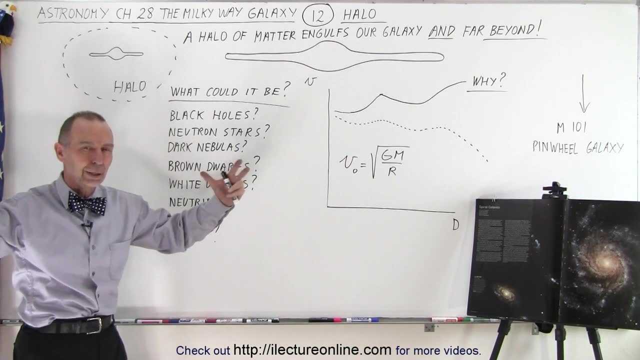 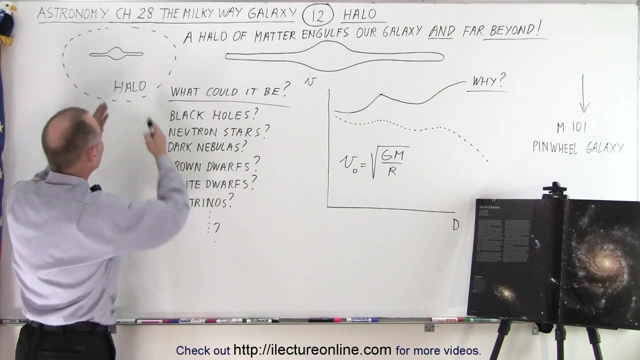 And we assume that the mass goes on way beyond the confines of the galaxy, a big halo of material that we can't see, And that's why we call it the halo. It's what engulfs the entire galaxy, permeates the galaxy. goes far out beyond the confines of the galaxy, As much as 300,000 light. 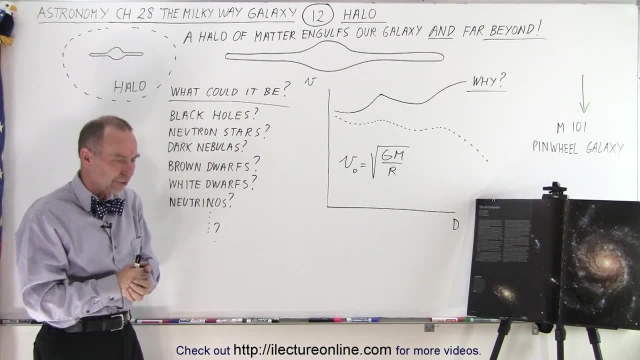 years across, when our galaxy is only about 100,000 light years across. What could it be? We don't know, We can't see it, we can't test for it, we can't detect it, but it must be there. There's matter. 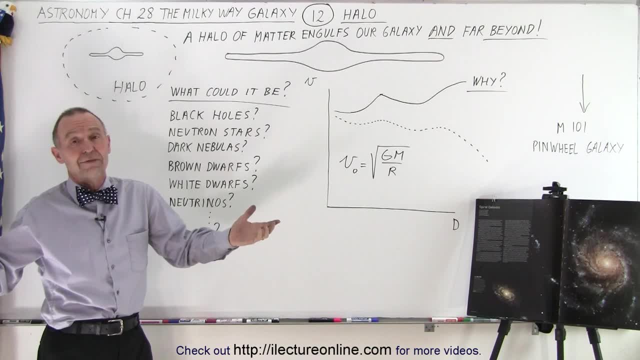 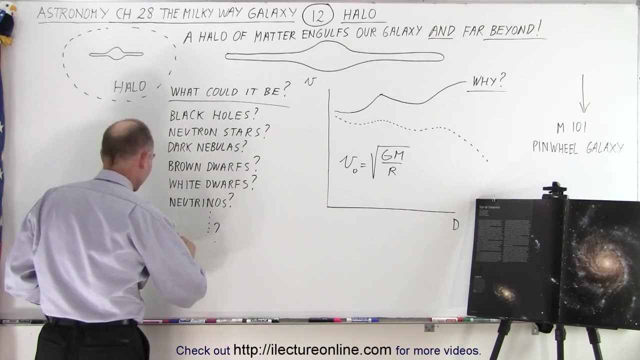 that is just not visible to us, And so the perfect name for it is dark matter. That's right. Dark matter is what we call it Now, just because we're not able to see it, we can't detect it, And so we're. 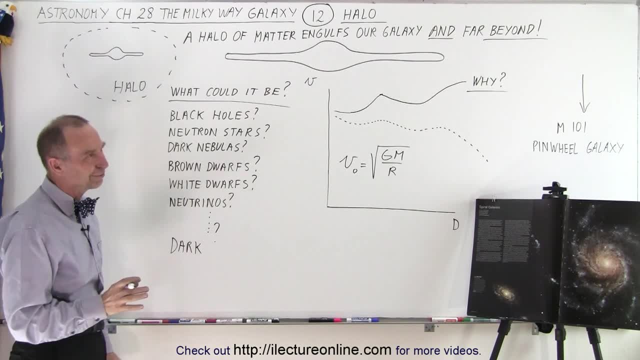 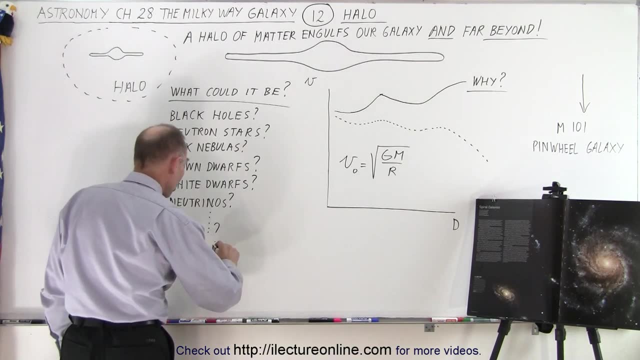 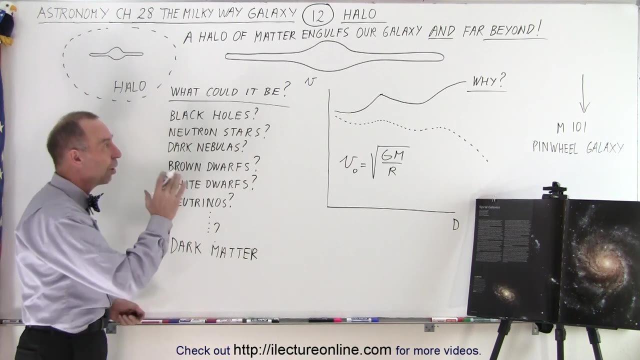 we give it a name, and that's the thing in science that always kind of puzzles me. It's almost like once we give something a name, it's like we know what it is, But it turns out we have no clue what dark matter could be. The reason why we call it matter, because it has to have mass, otherwise 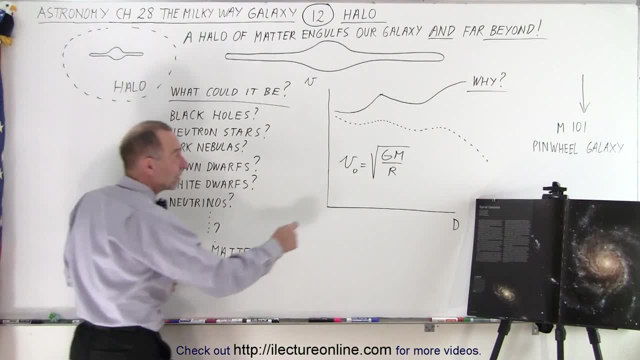 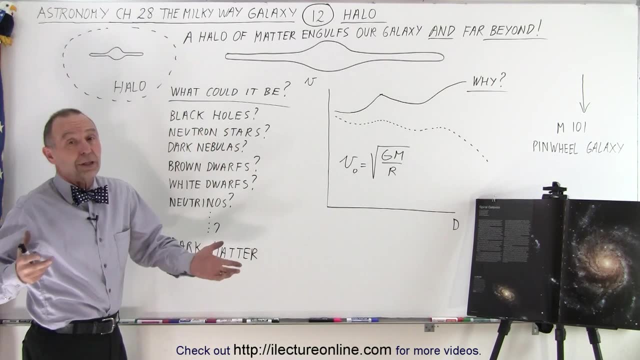 those stars would not be going as fast as they are. We need to account for that additional mass to give it a large enough velocity. We call it dark matter because it's dark. It doesn't give off any light. It doesn't give off any sort of electromagnetic radiation that we can detect. 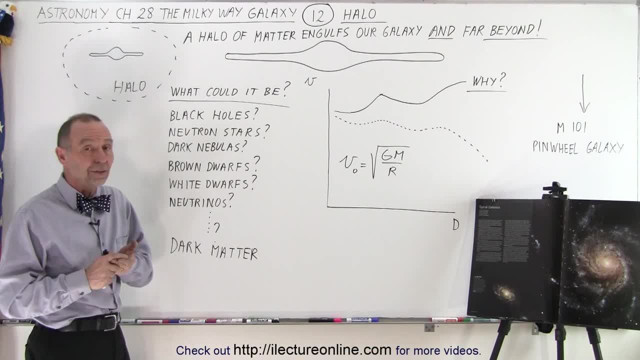 It's got to be there, It has to have mass, and we can't see it. So yes, dark matter is indeed a good name for it, And it turns out that by now we've estimated there must be at least five times as 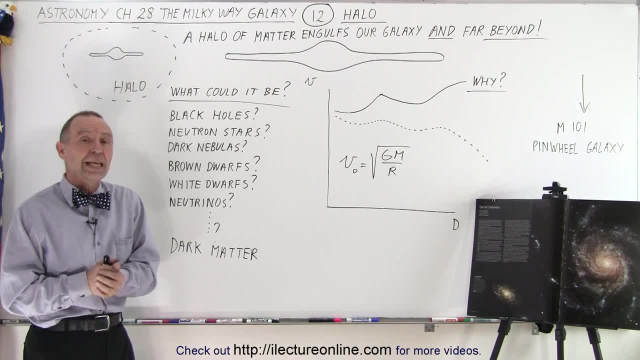 much mass in dark matter as there is in the visible matter of the galaxy. Five times as much. It's almost like five galaxies inside that halo that we can't see. Well, yes, It's got to be there, but what could it be? Some people even suggest it may be something that. 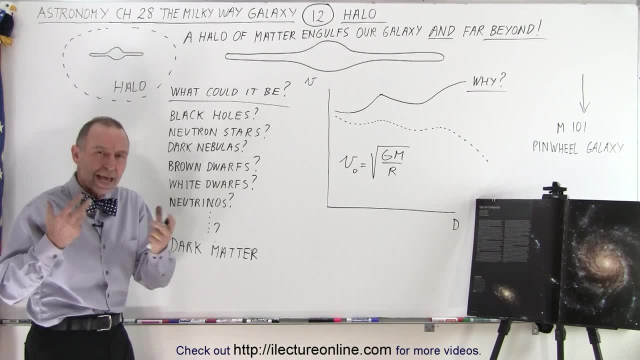 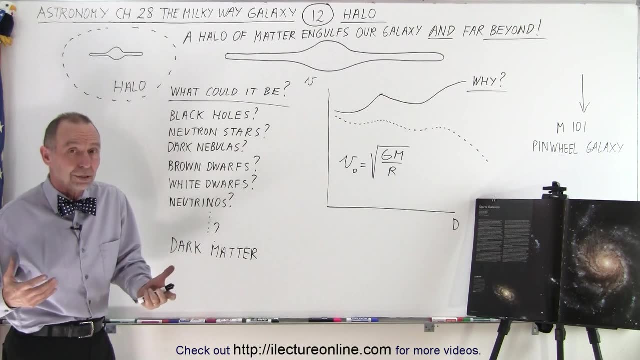 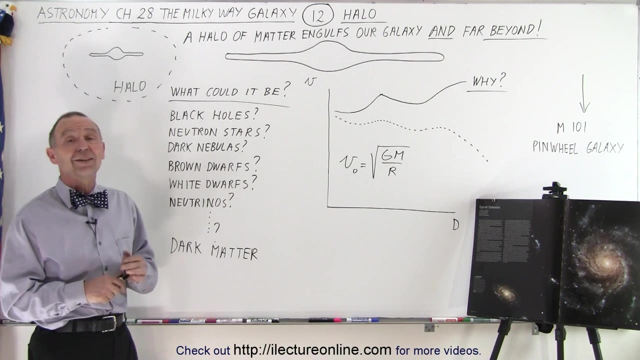 doesn't fit on the periodic table. a whole other type of matter that we cannot account for, that may not be made by protons and neutrons and electrons, that may be made by some other particle yet not discovered. It's a real mystery and we can't explain it, But it's got to be there. 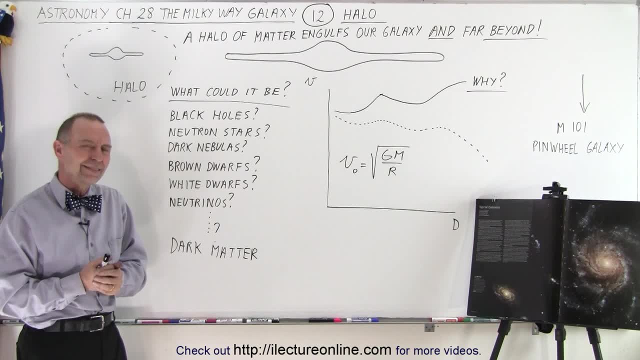 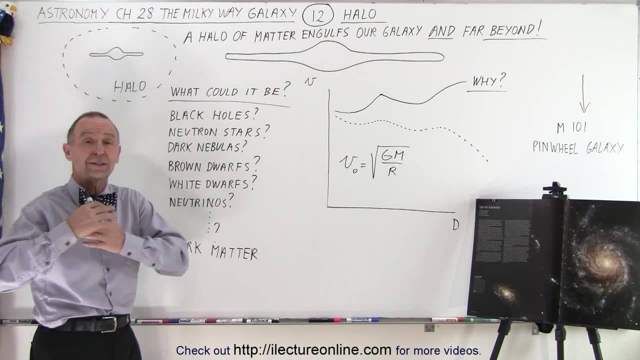 otherwise we cannot explain what's happening in our galaxy. It seems kind of odd, But you know what? We've been wrong before. We've thought certain things before and then later on we prove that they're not that way at all. It's something very different, Perhaps dark matter. 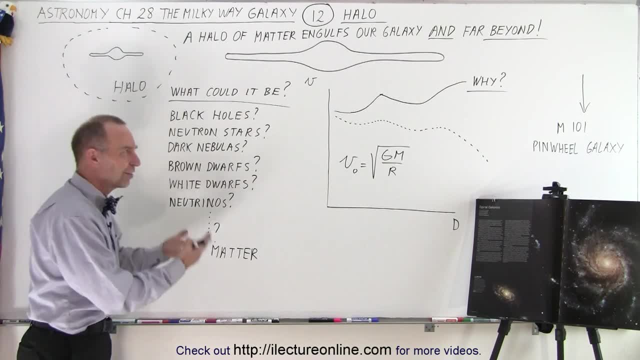 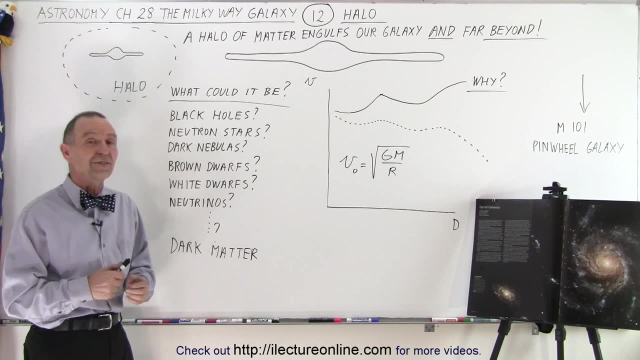 doesn't even exist. Something else exists, Something else explains it. We just haven't been able to explain it yet. Of course, that's not a popular thing to say, because many astronomers, many scientists, are absolutely convinced there must be such a thing as dark matter. 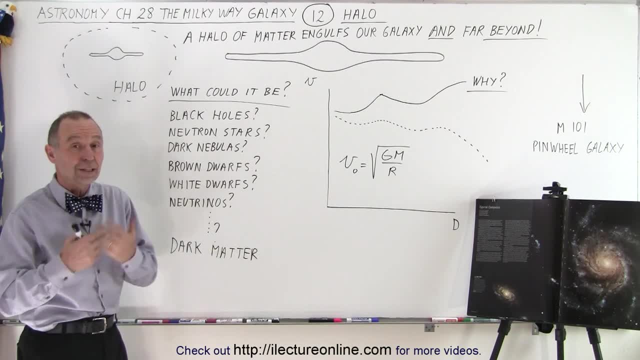 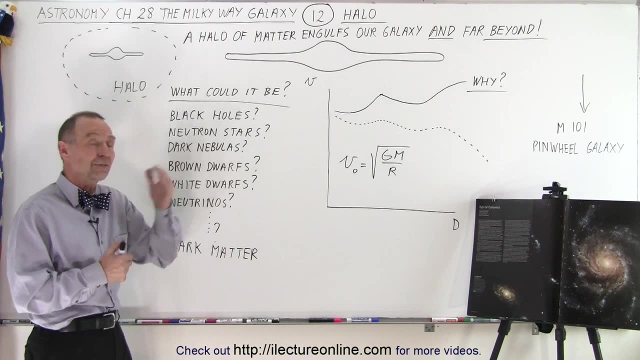 and they've calculated it. They've calculated how much of it must be and they've integrated it in the equations of cosmology and they think it explains some things we otherwise couldn't explain, like this, for example. So yes, it seems to be like there must be dark matter, but we have no. 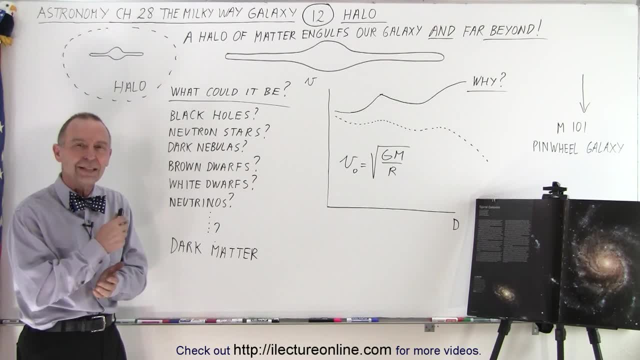 clue what it is. And that's the strange thing about it: We have not yet discovered what it is, although some people have theories, They've done some calculations, They've tried to figure out what it is. We just don't know yet what it is, But somehow something has to be there. 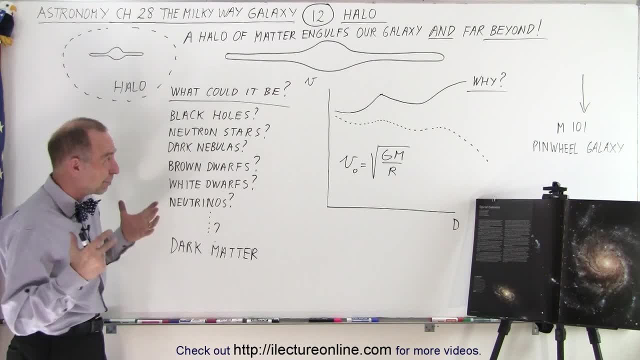 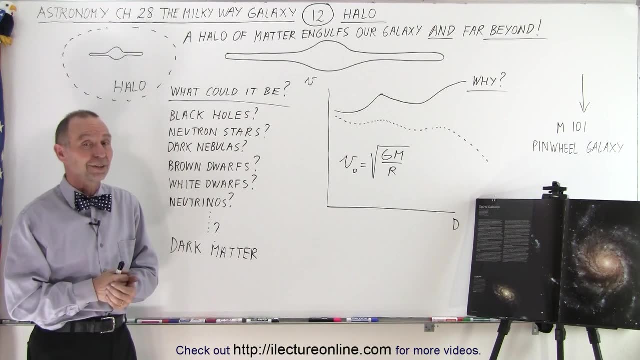 a halo, form of it surrounding our and permeating our galaxy. otherwise, we cannot explain this by the laws of physics. It's a real mystery. It still is. Could it be a different equation to explain it? Not a chance. That's the only equation. 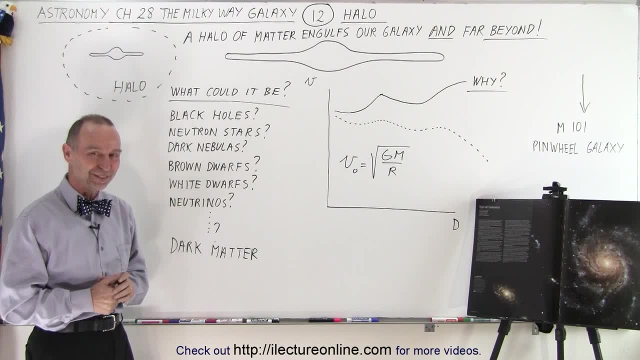 That's it. That's the equation. It has to fit that equation. That's the laws of physics. Or maybe there's something you overlook in the laws of physics? Not a chance. Quantum mechanics is…. Well, quantum mechanics is a different animal, Right? So these are the macro laws of physics. 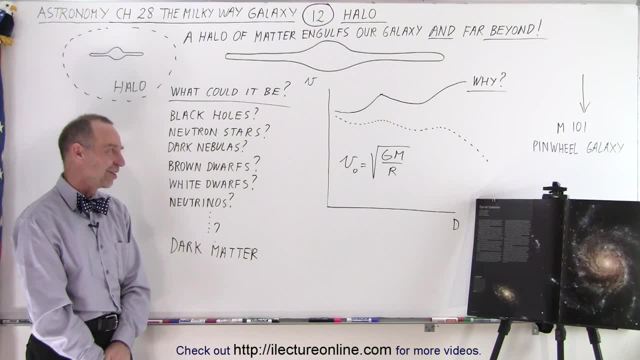 Those are very well established, very well understood. There's not a chance that we could overlook something. Something is driving the speed of those stars and those nebulas. Could it be a new thing in physics, A new branch? Nope, Nope, I don't think so. However, of course, if there is such a thing as dark matter, 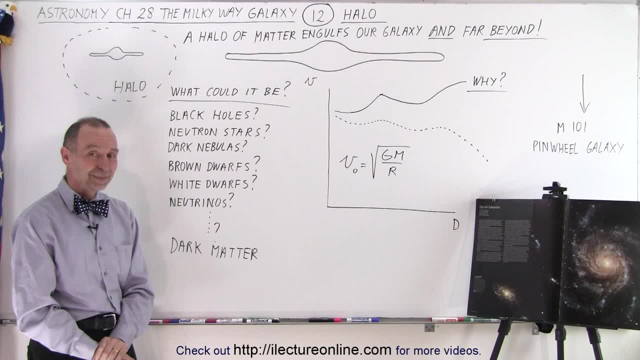 a new. it doesn't fit on the periodic table. it's made out of something different that we don't have, that we haven't discovered yet. that would be quite a discovery. I'm sure there's a Nobel Prize waiting for whoever figures out. but dark matter is well the Nobel Prize in science. that is all right. you. 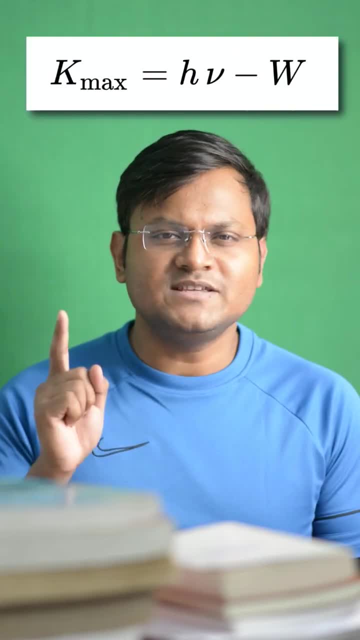 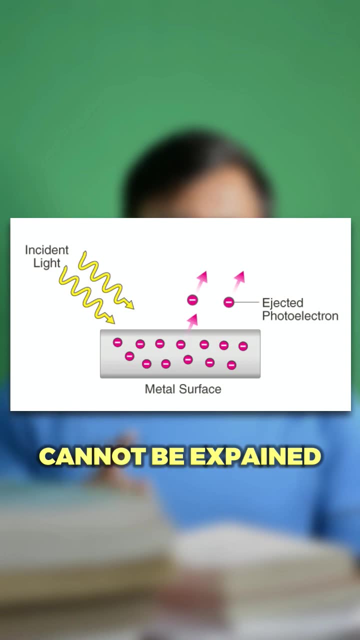 The birth of quantum mechanics and the Nobel Prize to Albert Einstein came from this simple equation of photoelectric effect. You see, when light strikes a metal surface, electrons are emitted. but this simple observation cannot be explained by classical physics. Back then, light was thought to consist of oscillating electric and magnetic fields. The energy of 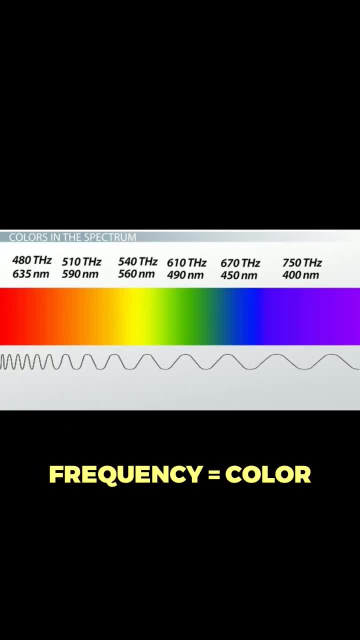 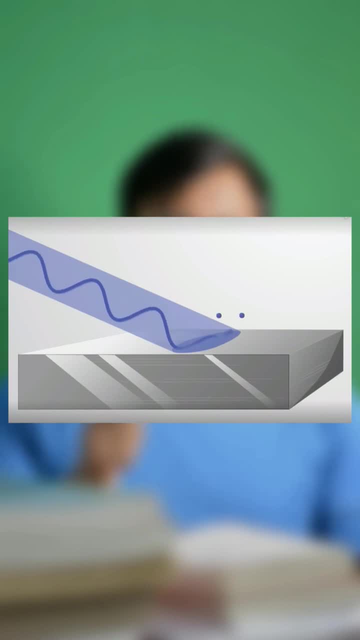 these oscillations depends upon the intensity of light, and the frequency only decides the color. Based on this wave theory, even if a low intensity of light falls on a metal surface, electrons should be emitted. even if it took hours, days or weeks, But it was. 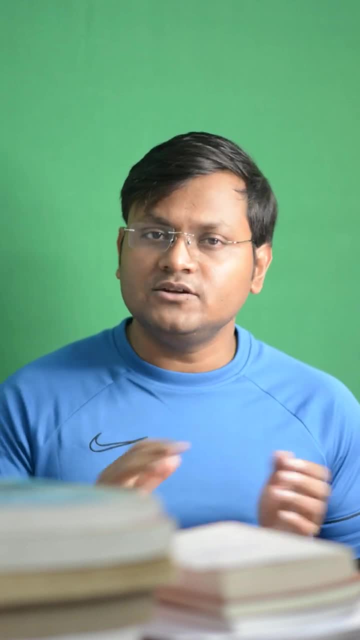 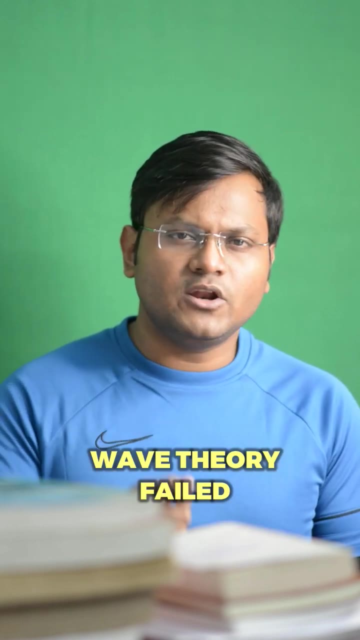 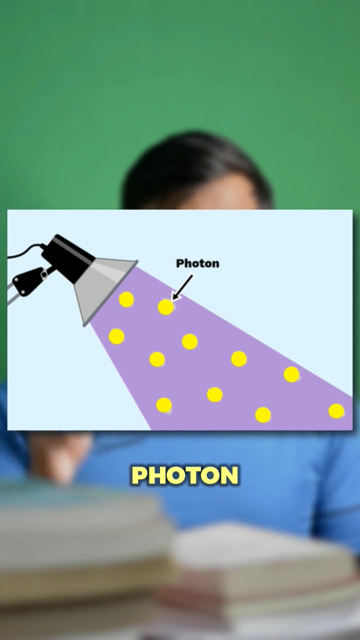 found that photoelectric emission is an instantaneous process that has nothing to do with the intensity and everything to do with the frequency of light above a certain threshold. Wave theory failed to explain this simple phenomena, so Einstein came up with the revolutionary idea that light is not a wave but a particle, a photon, whose energy is decided by its frequency. 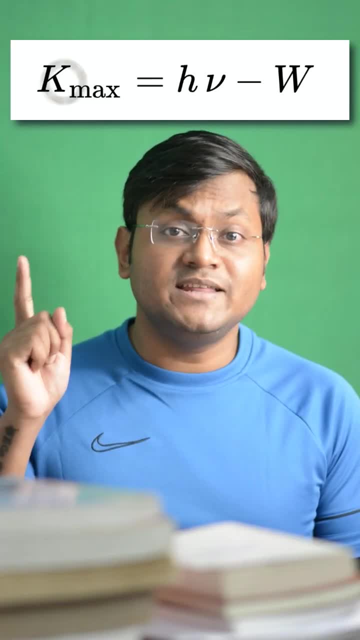 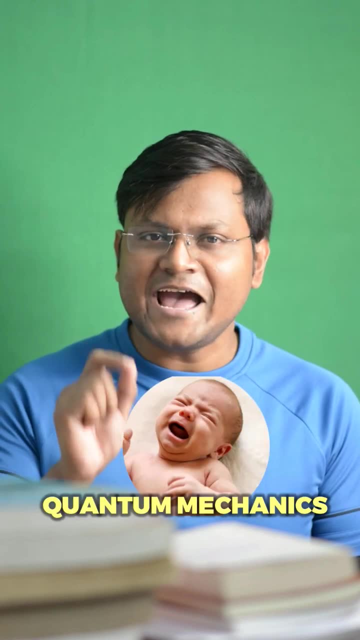 and it has nothing to do with intensity. He provided a very simple equation: that the energy of the emitted electron is equal to the energy of a photon, minus the work function. The success of this equation gave birth to quantum mechanics and the Nobel Prize in physics. 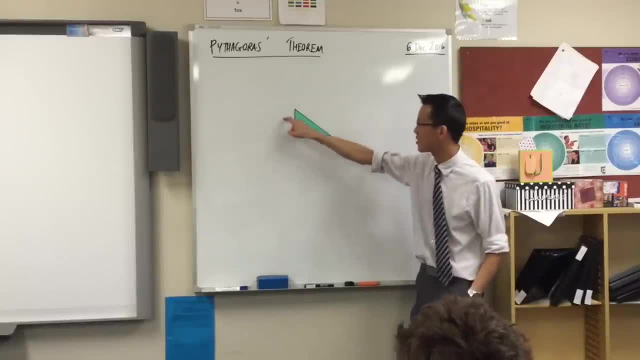 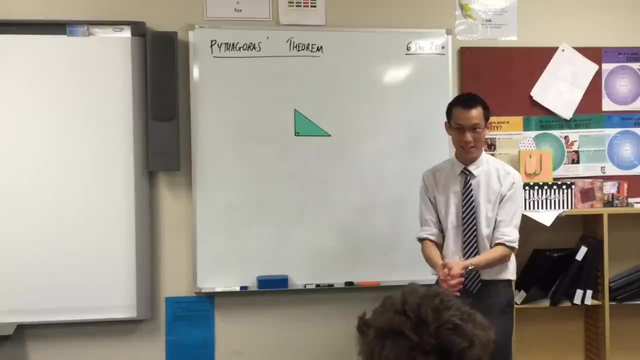 I will tell you what the theorem is in a minute. It has something to do with how all of the sides of this triangle relate to each other. I'm going to show you what the result is, but I want to show you how I get the result. 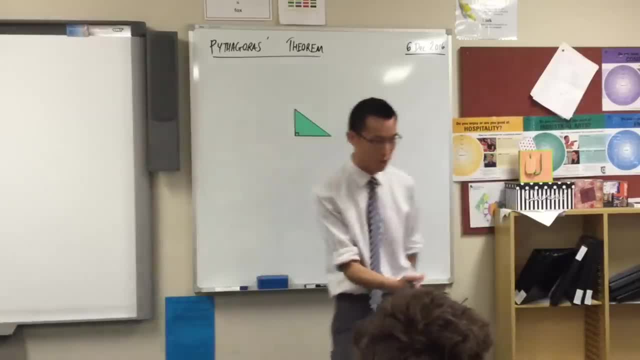 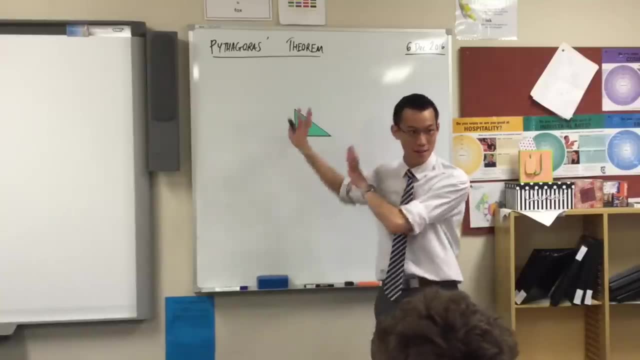 So all of this that I'm about to do on the board, you will have your time to draw. I actually have a little guide for you that I'm going to put up on the screen in a minute, But for now I just want you to be fully engaged, with your eyes on what's happening here.